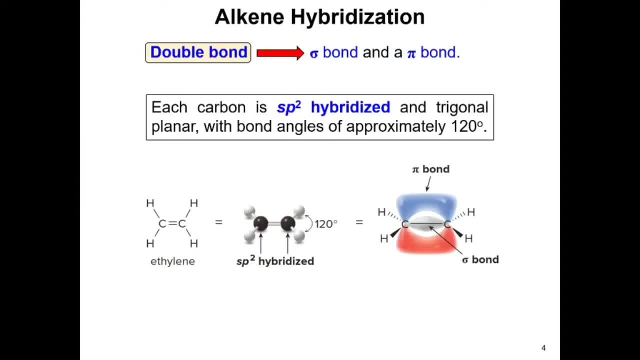 So, if you remember, a carbon-carbon double bond contains two different types of bonds: a sigma bond and a pi bond, according to the valence bond theory. In this theory, both carbon atoms that are involved in the double bond are sp2 hybridized. 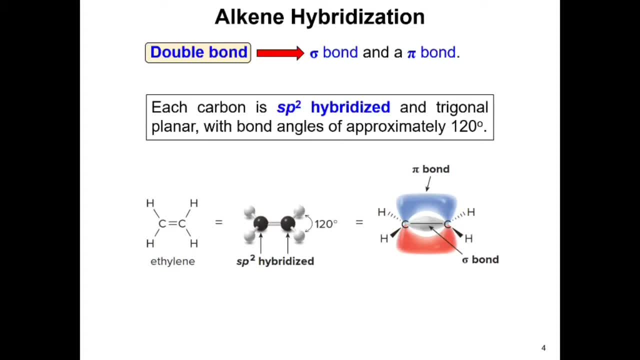 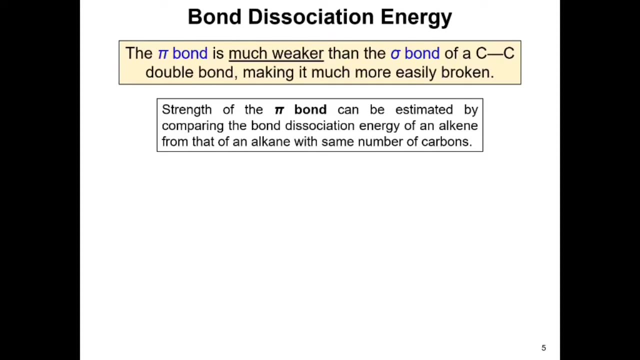 with a trigonal planar geometry and bond angles of about 120 degrees. The pi bond is oriented above and below the plane, whereas the sigma bond is oriented within the plane. In terms of energy, pi bonds are actually weaker compared to sigma bonds within the same 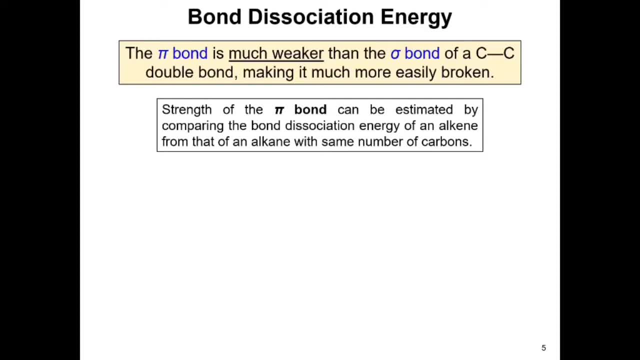 carbon-carbon double bond, And that's why they're a lot easier to break compared to sigma bonds. The strength of the pi bond can easily be estimated by comparing the bond dissociation energy of an alkene from that of an alkane with the same number of carbon atoms. So let's take a look at ethylene. 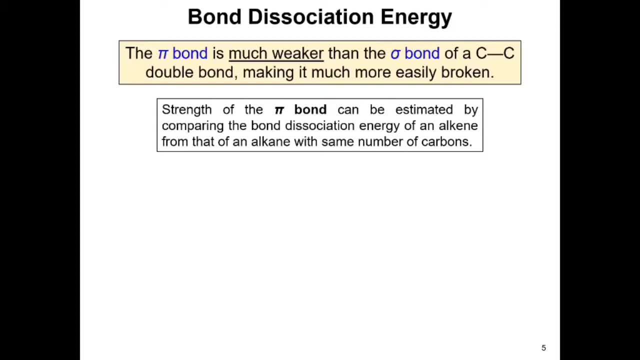 and ethane, for example. They both have the same number of carbon atoms. the only difference is one contains a pi bond and the other doesn't. So here you can see that it would require 635 kilojoules per mole of energy to break this double bond in ethylene, Whereas in ethane. 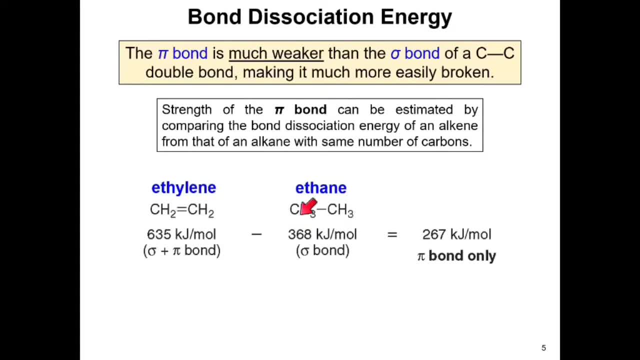 it would only require 368 kilojoules per mole of energy to break this double bond in ethylene. And if we take the difference between the two energies here, we get the energy of the pi bond only, And you can see that this energy is less compared to the energy of the sigma bond. 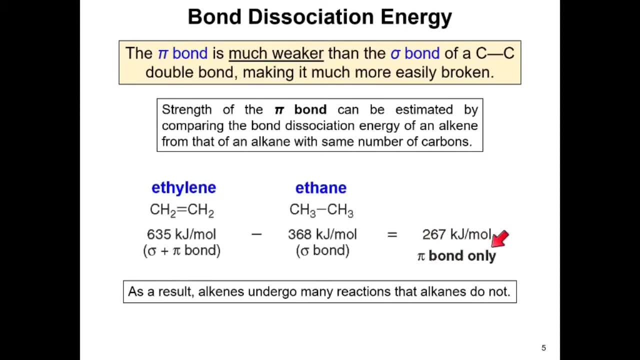 And that's why pi bonds are easily broken in a lot of chemical reactions, And so this is one of the main reasons why alkenes undergo many reactions that alkanes do not, In terms of alkenes within a ring, cycloalkenes with less than 8 carbon atoms, actually prefer. 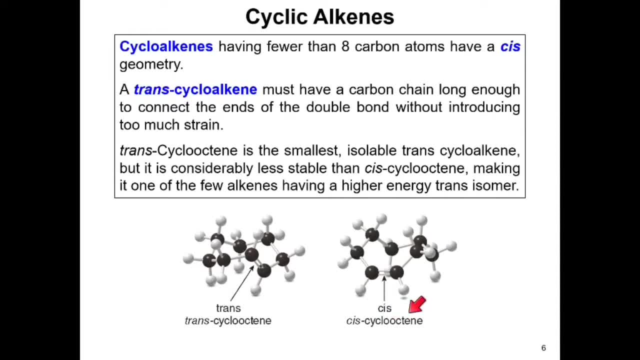 cis geometry. So here we have cis cyclooactene with 8 carbon atoms. You can see that we have a cis geometry here, because the two carbon atoms are on the same side of the double bond, Whereas in trans cyclooactene the two carbon atoms are on the opposite sides of the double bond. 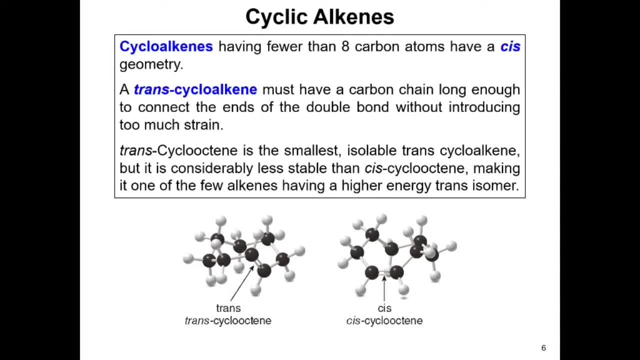 So that means that cycloalkenes with less than 8 carbon atoms are more stable having a cis geometry than trans geometry, must have a carbon chain long enough to connect the ends of the double bond without introducing too much strain, And so the trans-cyclo-octene is actually the smallest isoluble trans-cyclo-alkene. 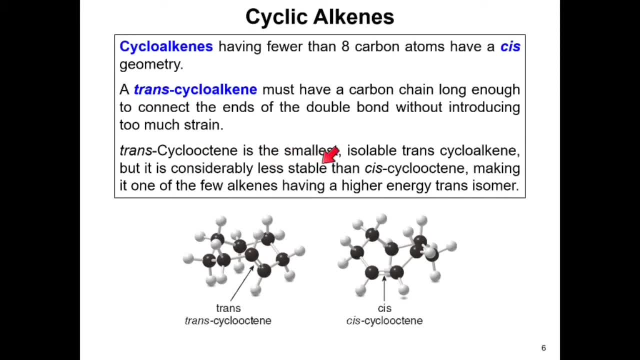 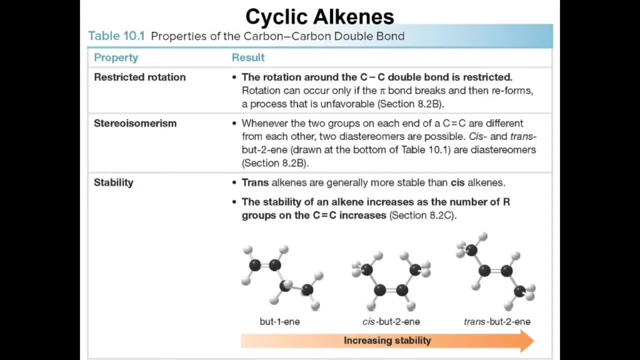 but it's still actually considerably less stable compared to a cis-cyclo-octene, making it one of the few alkenes having a higher energy trans-isomer. So here's a table that basically summarizes the different properties of the carbon-carbon double bond. So you already know that double bonds have 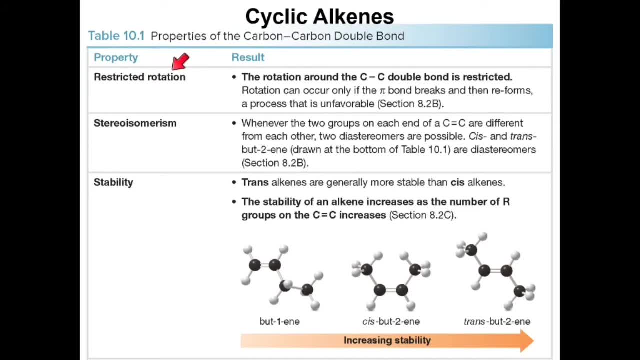 restriction on their rotation, and the reason why is because of the presence of the pi bond. So the only time that you can rotate around a double bond is if you were to break that pi bond, In terms of stereoisomerism, whenever you have two different groups on each end of the double bond. 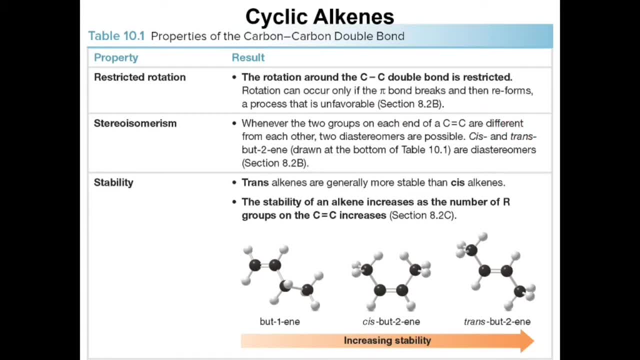 then a cis and trans isomers are possible, And in terms of stability, the more substituted the double bond is, the more stable they are, And so the stability of an alkene increases, and the more stable they are, And so the stability of an alkene increases. 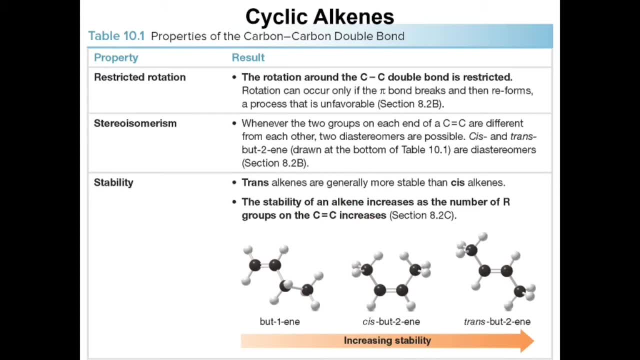 and the more stable they are, And so the stability of an alkene increases as the number of R groups on the double bond increases, And also generally, trans-alkenes are more stable compared to cis-alkenes And again, the only exception here is if you have a cycloalkene. 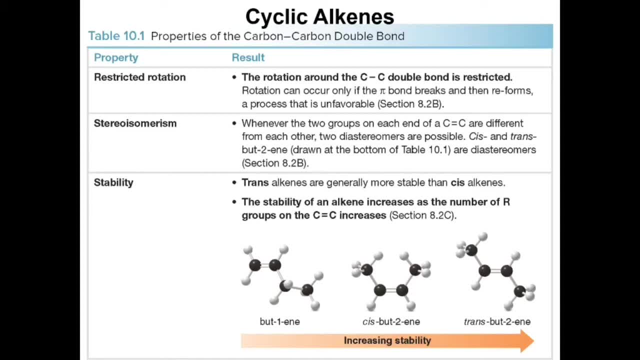 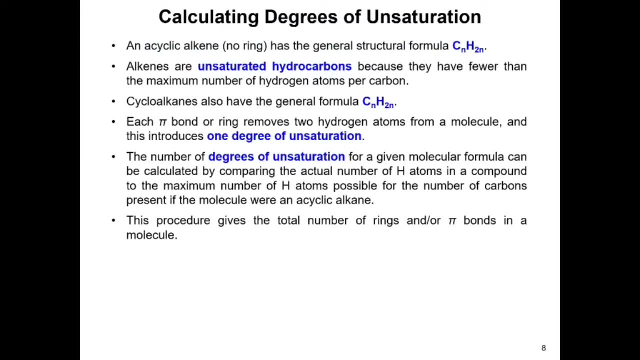 with less than eight carbon atoms. In that case the cis geometry dominates, So the degrees of unsaturation of a molecule can basically help us identify and predict whether its structure contains a pi bond, a cyclic ring or a combination of both. So for the first three bullet points here you should already know. regarding alkenes, 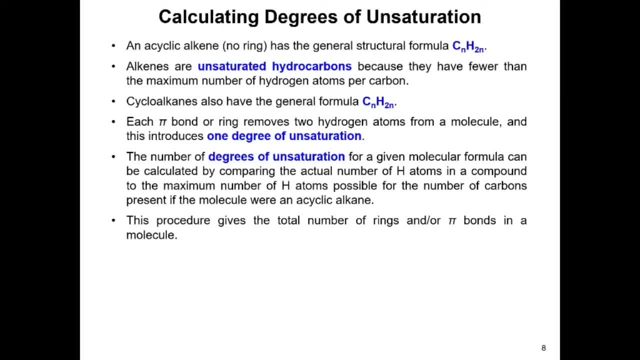 An acyclic alkene has the general formula CnH2n, So that means that you have two hydrogen atoms per carbon atom, And so if you have a total of five carbon atoms within the alkene, then that means that you have a total of 10 hydrogen atoms. Alkenes are considered unsaturated hydrocarbons. 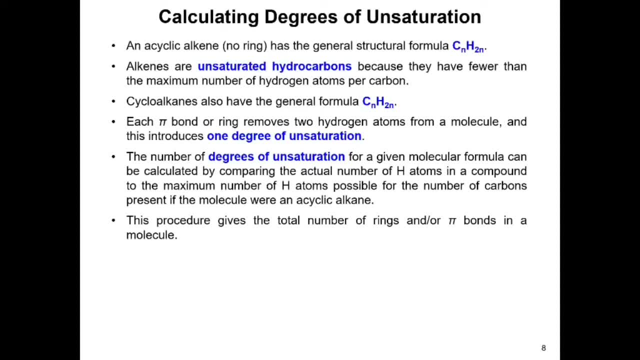 because they have less than the maximum number of hydrogen atoms per carbon. Cycloalkenes also have the same general formula as an acyclic alkene, which is CnH2n. So you can see here that both acyclic alkenes and cycloalkenes have two hydrogen atoms less compared to a saturated alkene with the. 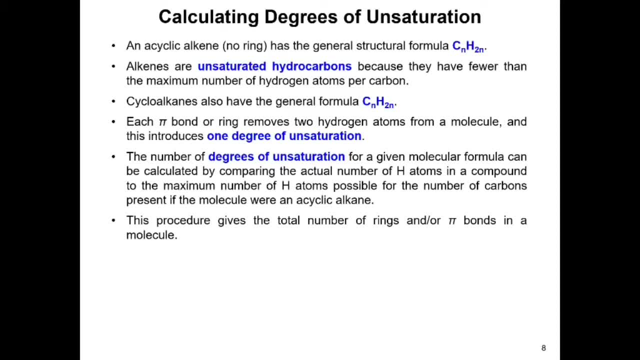 same number of carbon atoms. That means that each pi bond or ring removes two hydrogen atoms from a molecule, and this introduces one degree of unsaturation. So how do we determine the number of degrees of unsaturation for a given molecular formula? Well, we can calculate that by simply comparing the actual number of hydrogen atoms of that compound. 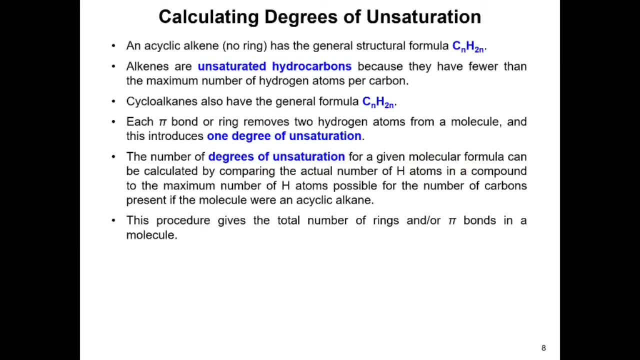 to the number of hydrogen atoms of a saturated alkene with the same number of carbon atoms. And once we've identified the number of degrees of unsaturation for a given molecular formula, then we'll be able to know the total number of rings and or pi bonds within that molecule. So 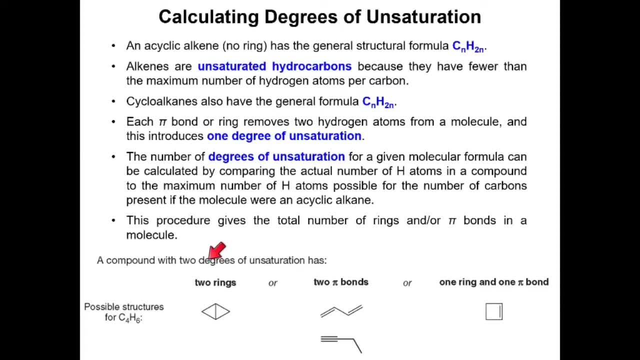 if a compound contains two degrees of unsaturation, that means its chemical structure contains either two rings or two pi bonds. So if a compound contains two degrees of unsaturation, that means two pi bonds or a combination of one ring and one pi bond. So here's an example, Calculate. 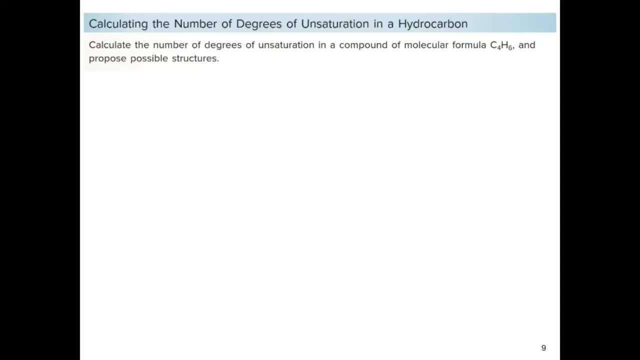 the number of degrees of unsaturation in a compound of molecular formula C4H6 and propose possible structures. So, in order to calculate the number of degrees of unsaturation, the first thing that we want to do is to determine the maximum number of hydrogen atoms in a saturated 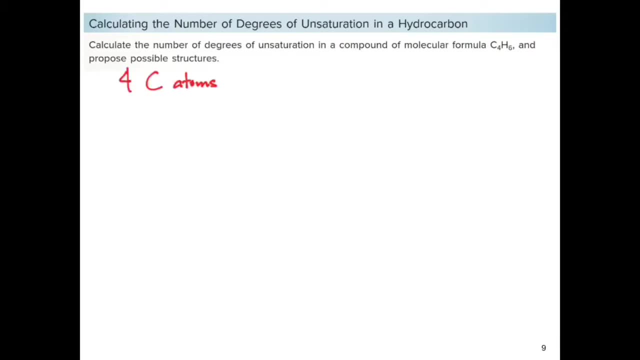 alkene with the same number of carbon atoms, And so, since we have four carbon atoms, that we have two n plus two, in which n is the total number of carbon atoms, And so substitute that for n. so two times four is eight plus two, and we get a total of 10 maximum hydrogen atoms. 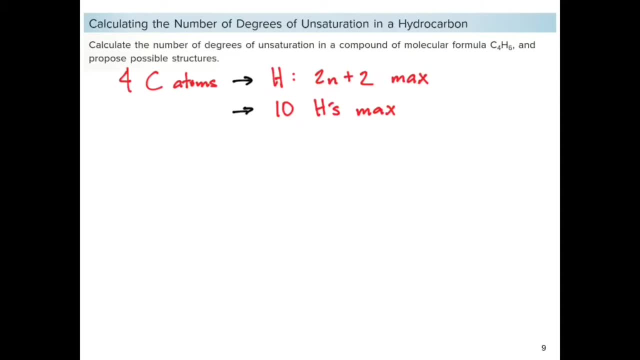 And so now, to calculate the number of degrees of unsaturation, all you have to do is take the difference between the maximum and the actual number of hydrogen atoms. So let's see how we can atoms, and then divide that by two. So here we have two degrees of unsaturation. So since we 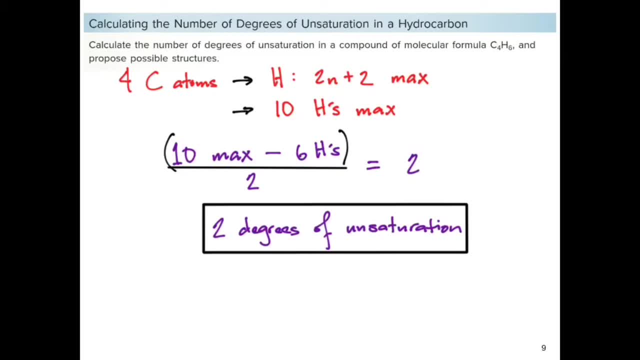 have two degrees of unsaturation. there are three possible structures here. The structure can have two rings, It can contain two bonds or two pi bonds or a combination of the two. So one ring and one pi bond. And for the first one here we can have two rings with four carbon atoms and six. 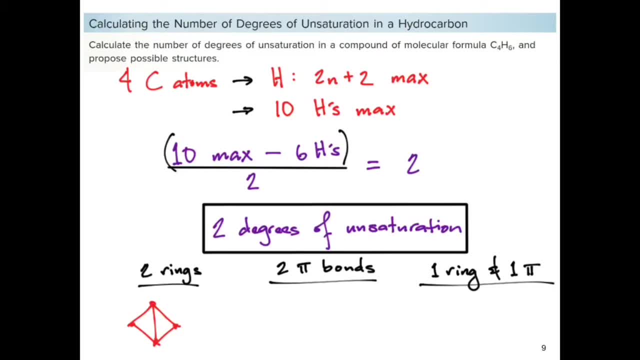 hydrogen atoms, And then for the second one we can have two pi bonds. We can have two possible structures. You can see that we have two pi bonds here, with a total of four carbon atoms and six hydrogen atoms, And the second structure here, this triple bond, contains two pi bonds as well. 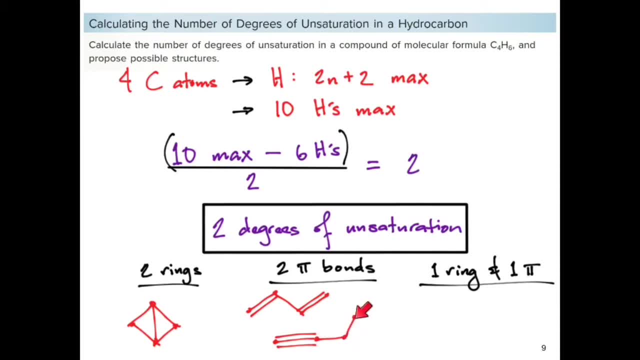 And you can see that it contains a total of four carbon atoms and six hydrogen atoms, And then, finally, we can have a ring and a pi bond. So it's a combination of a ring and a pi bond. So you can see that we have four carbon atoms here. 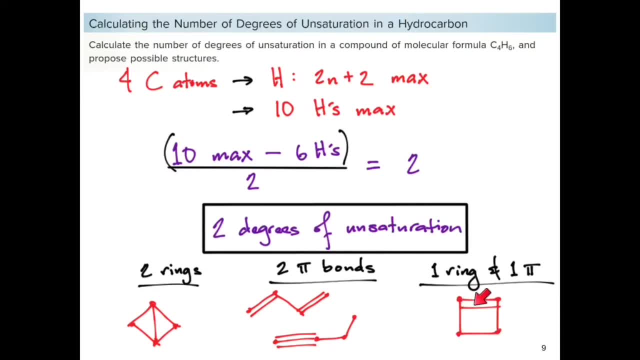 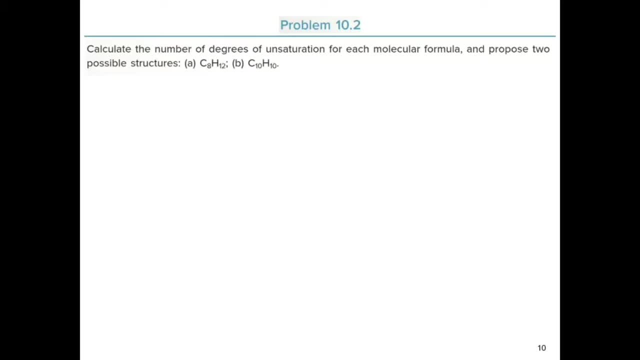 in a ring and contains a pi bond. Here's practice. problem number two: Calculate the number of degrees of unsaturation for each molecular formula and propose two possible structures. So for the first one, here we have C8H12.. So we have a total of eight carbon atoms. 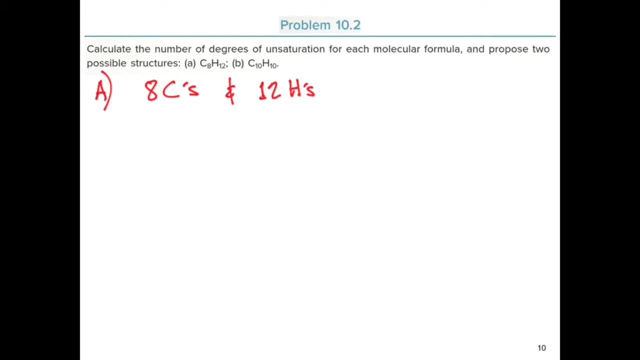 and 12 hydrogen atoms, And so we can calculate the number of degrees of unsaturation by calculating or determining the maximum number of hydrogen atoms possible per carbon atom. And so if we have eight carbon atoms, we can use this formula here to calculate the maximum number. 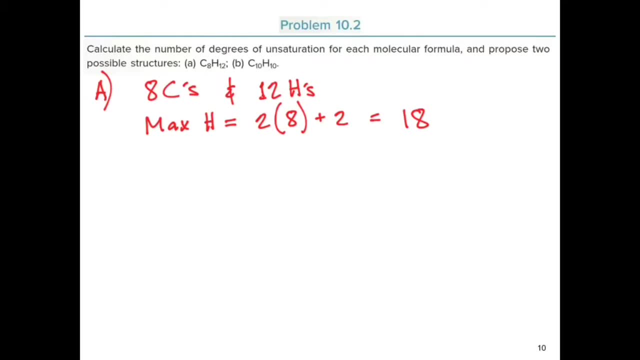 of hydrogen atoms, And so two times eight plus two and we get 18 maximum hydrogens. And so now we can take the difference between the maximum and the actual number of hydrogen atoms divided by two, And if we do that we get three degrees. 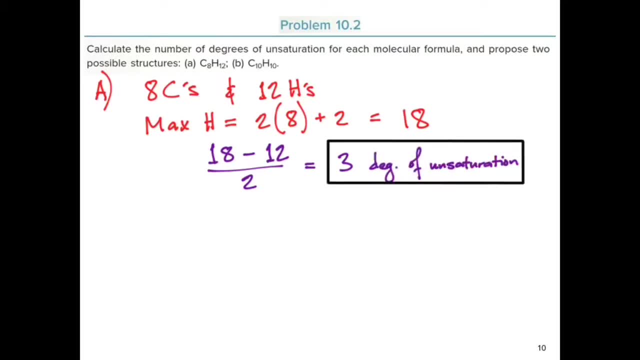 of unsaturation. So for the first one we can have three rings. So you can see that we have a total of three rings here, And when you count the total number of carbon atoms and the number of hydrogen atoms, it checks out All right. And we can also have one ring and two pi bonds within the. 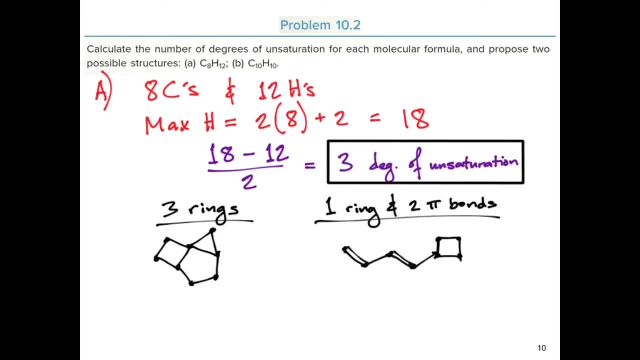 structure. So here's a ring and two pi bonds, So you can have two double bonds here and a ring containing four carbon atoms. So again, when you count the total number of carbon atoms here and hydrogen atoms, it should equate to eight carbons and 12 hydrogens. 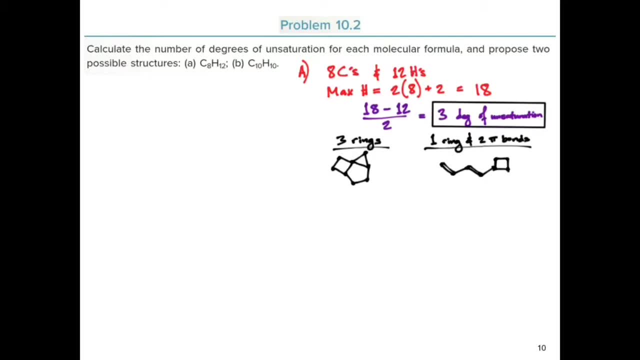 So for the next one, here we have C10H10. And so we have a total of 10 carbon atoms and 10 hydrogens. So the very first step here is to calculate the maximum number of hydrogens for the same number of carbon atoms. And so two times 10 carbon atoms plus two, and we get 22. 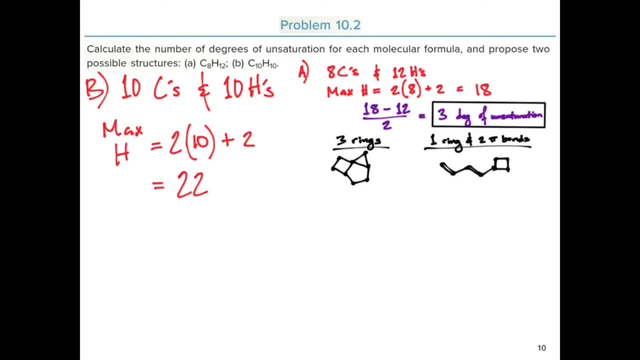 maximum hydrogens possible. And so now we can take the difference between the maximum and the actual number of hydrogen atoms divided by two, and we get six degrees of unsaturation. And so with six degrees of unsaturation we can have a structure with six pi bonds. You can have six rings or a combination. 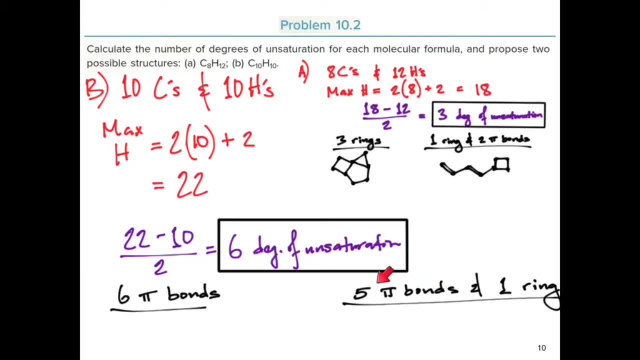 of pi bonds and rings. So I chose five pi bonds and one ring. So with six pi bonds you can get bonds. you can have this structure shown here so you can have a combination of double bond and triple bonds. so this triple bond here contains two pi bonds. so we have two, three, four, five, six. 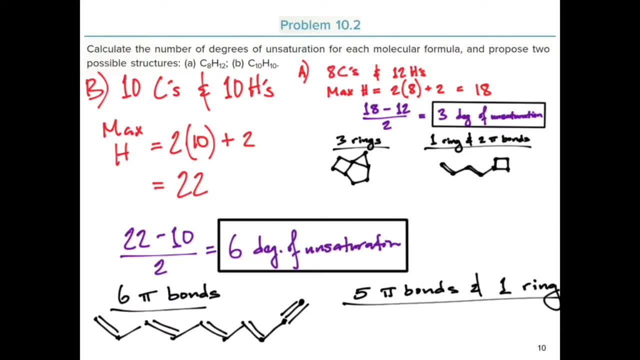 pi bonds and again you can count the number of carbons and hydrogens, and it should equate to 10 carbons and 10 hydrogens. and for the second structure here we can have five pi bonds and one ring, and so this structure here shows you a ring with three pi bonds plus two pi bonds outside the 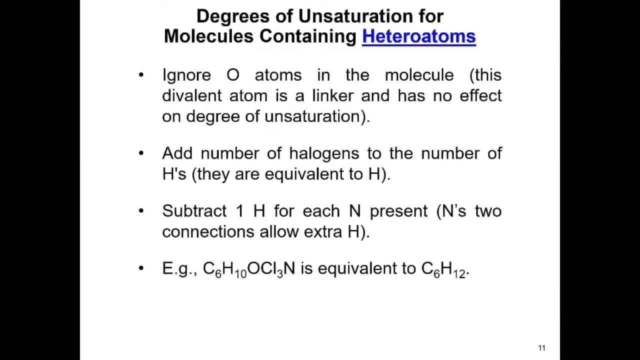 ring? and what about for molecules containing heteroatoms? how do we calculate the degrees of unsaturation for these molecules? so here are some of the steps that you can follow in determining or calculating the degrees of unsaturation for these kind of molecules. when it comes to oxygen, 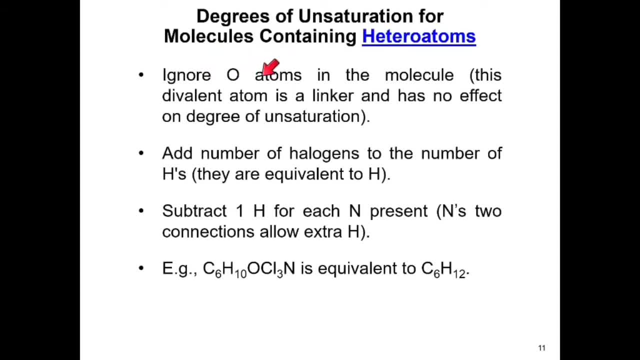 atoms. ignore them. ignore the oxygen atoms. they have no effect you on the degree of unsaturation. when it comes to halogens, add the number of halogens to the number of hydrogens, so they're essentially equivalent to hydrogen atoms. when it comes to nitrogens, 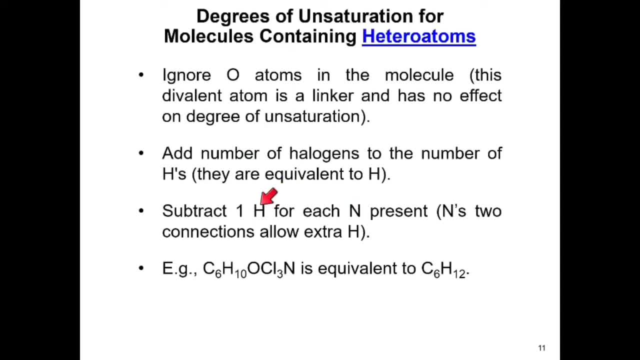 you're going to subtract one hydrogen for each nitrogen present, and so here's an example: we have c6, h10, ocl3 nitrogen, so you can see that we have 10 hydrogens here. we're going to ignore that, the oxygen atom, and then add three to the existing. 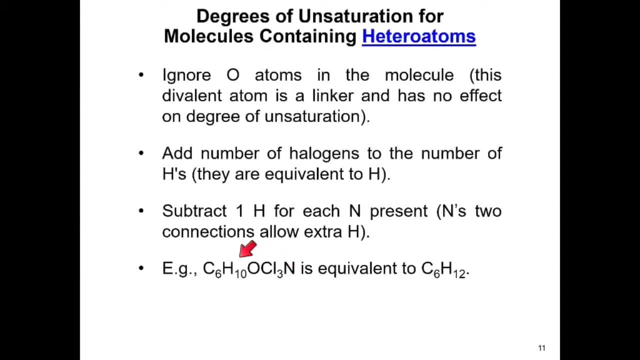 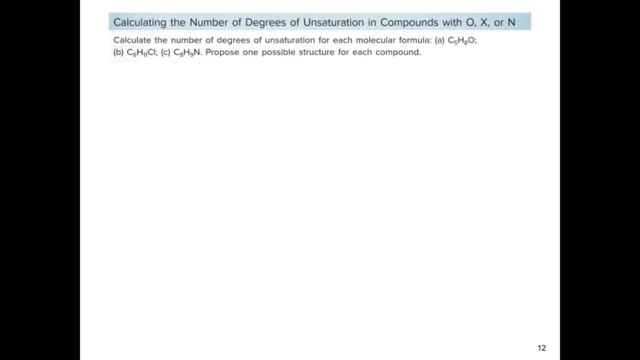 ten and it subtract one because of the nitrogen. so this molecule has essentially the same degrees of unsaturation as C6H12. so here's an example: calculate the number of degrees of unsaturation for each molecular formula. so for the first one, here we have c5H8O, so we have a total of five. 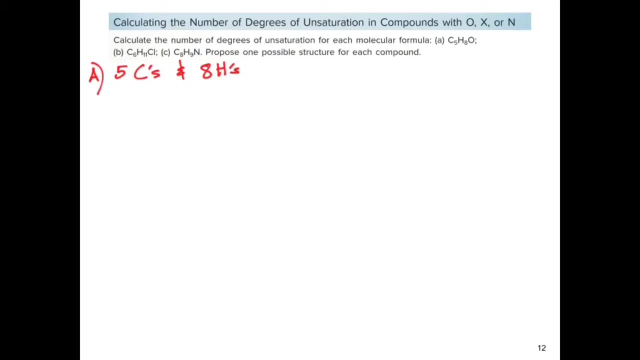 carbons and eight hydrogen atoms. so for the oxygen atom, we can ignore this, because he has no effect on the number of degrees of unsaturation. And so again, the very first step here is to determine the maximum number of hydrogen atoms possible for five carbons. And so 5 times 2 is 10, plus 2 equals 12.. So the 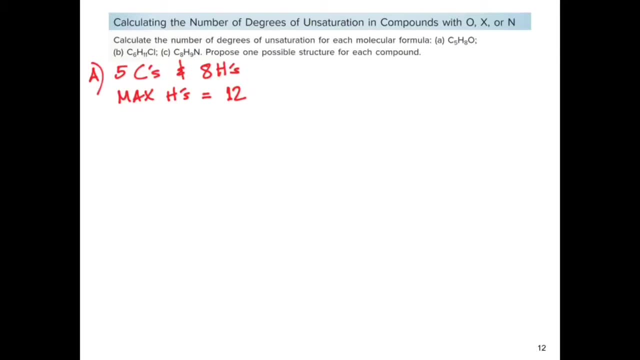 maximum is 12 hydrogens, And then we're going to take the difference between the maximum and the actual number of hydrogen atoms divided by 2.. So 12 minus 8 divided by 2 equals 2.. So that means we have 2 degrees of unsaturation, And so the structure should contain either two rings: 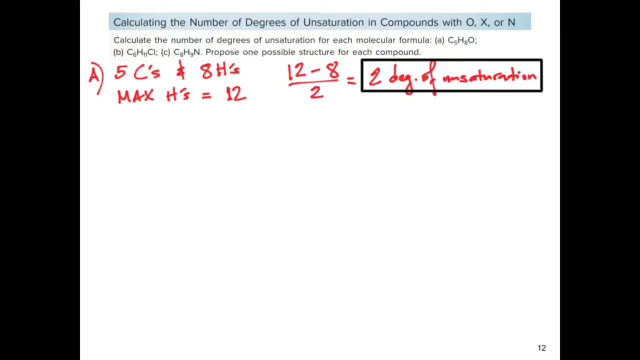 two pi bonds or a combination- one ring and one pi. So here's the one that I chose. The oxygen atom is part of the ring And you can see that we have a total of 1,, 2,, 3,, 4, 5 carbon atoms. 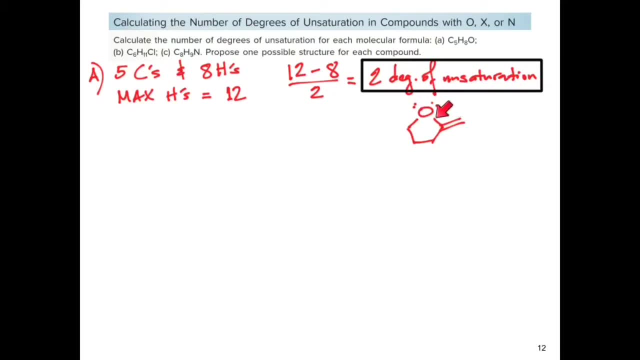 with one double bond or one pi. So a ring and a pi would count as 2 degrees of unsaturation. And so the structure should contain either 2 rings, 2 pi bonds or a combination: 2 degrees of unsaturation. And for the second one here we have C6, H11, and 1 chlorine. So we 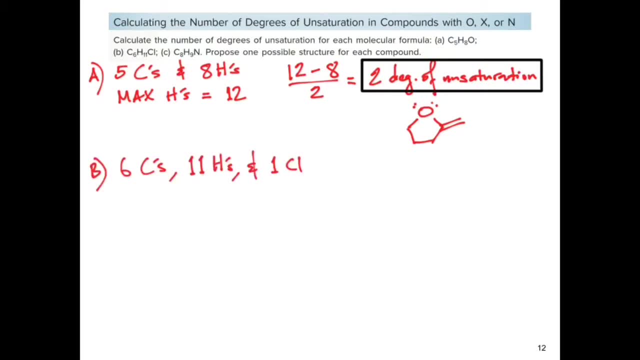 have 6 carbon atoms, 11 hydrogens and 1 chlorine atom, And so we're going to count 1 chlorine as 1 hydrogen, And so that means that we have 12 hydrogens total here, And so again we're going. 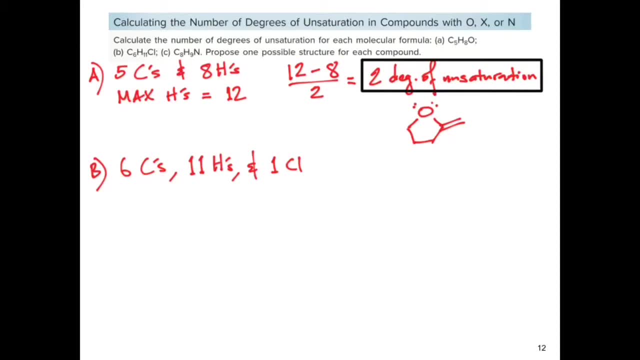 to count or calculate the maximum number of hydrogens possible for 6 carbon atoms. 6 times 2 is 12, plus 2 equals 4.. And so we're going to count or calculate the maximum number of hydrogens: 14.. So 14 maximum hydrogens. And then we're going to take the difference here, 14 minus 12 divided. 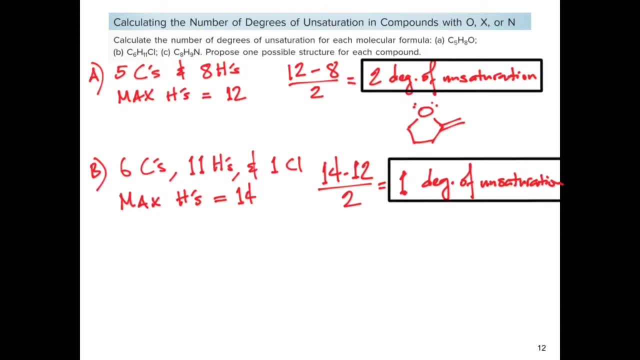 by 2 equals 1.. And so for this specific molecule we only have 1 degree of unsaturation, And so you can draw, we can use this structure right here, which is basically cyclohexane with a chlorine attached to the ring, And so we have 1 ring here which counts as 1 degree of unsaturation, And for 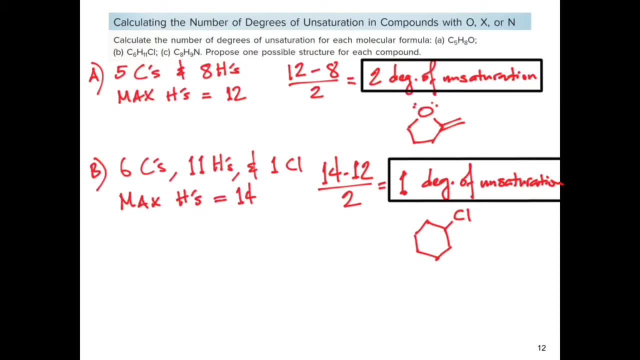 the third one. here we have C8, H9, and 1 nitrogen, So we have 8 carbons, 9 hydrogens and 1 nitrogen. So we have to subtract 1 hydrogen for every 1 nitrogen present, And so that means that 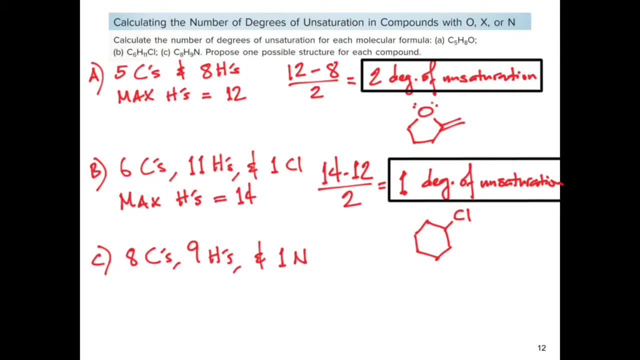 we have a total of 8 hydrogens here, And for the maximum number of hydrogens there's 18, because we have 8 carbons. 8 times 2 is 16, plus 2 equals 18.. And now we're going to take the difference. 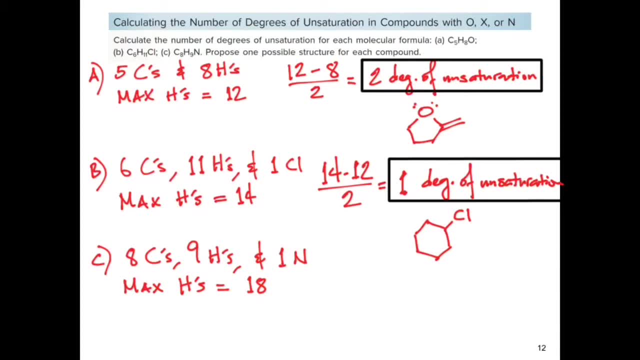 here. So 18 minus 8 equals 10, divided by 2, we have 5.. So we have 5 degrees of unsaturation for this molecule. So here's the structure: with 5 degree of unsaturation We have a nitrogen within. 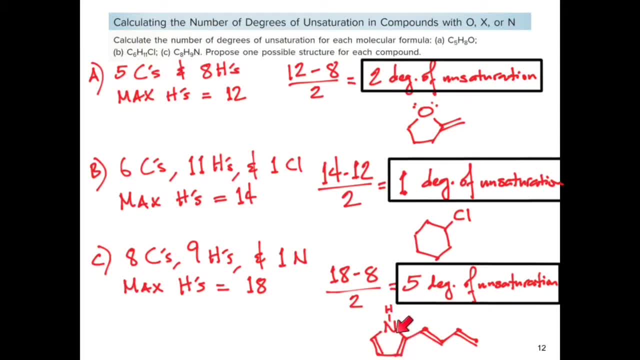 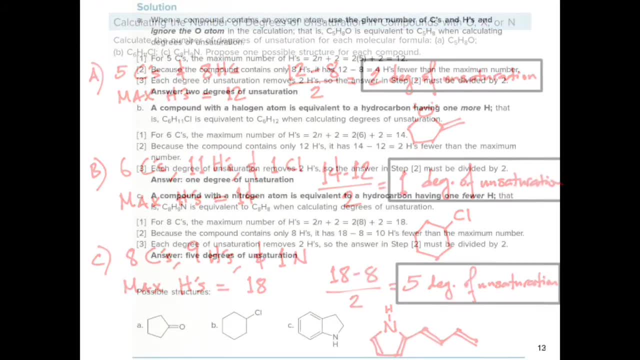 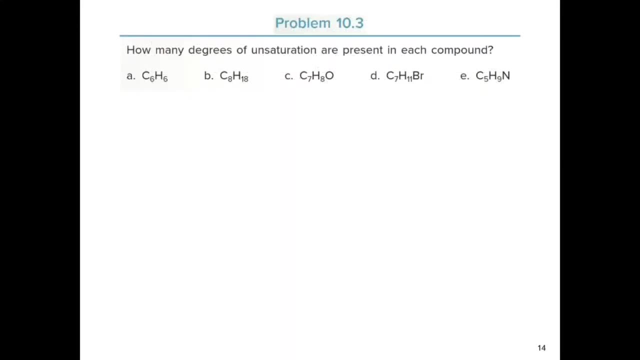 the ring. So 1 ring is 1 degree of unsaturation And then a total of 1,, 2,, 3,, 4 pi bonds, So that's a total of 5 degree of unsaturation. So here's practice problem number 3.. How many degrees of unsaturation are present in each? 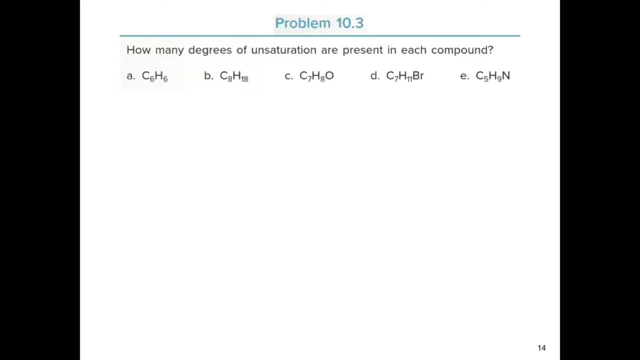 compound. So for the first one here we have C6, H6. So we have 6 carbon atoms and 6 hydrogens, And so the maximum number of hydrogens possible for this compound with 6 carbons is 6 times 2. 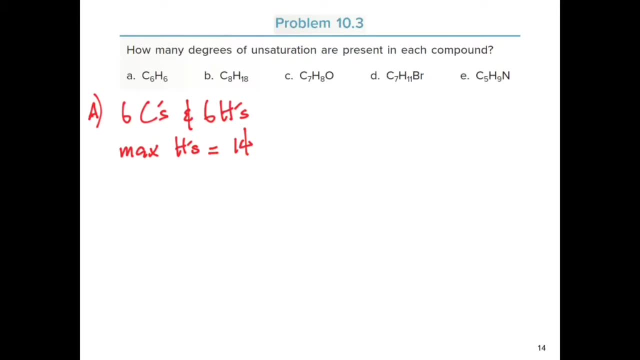 equals 12, plus 2 equals 14.. So we have 14 hydrogens maximum possible, And so the next step here is to take the difference between the two numbers here: 14 minus 8, and 2.. So we have 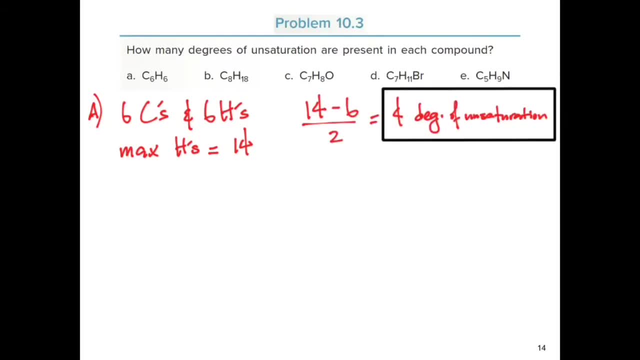 14 minus 6, and then divide that by 2.. So 14 minus 6 divided by 2, and we get 4 degrees of unsaturation. And for the next one here, part B, we have C8, H18.. So we have 8 carbon atoms and 18 hydrogen atoms. 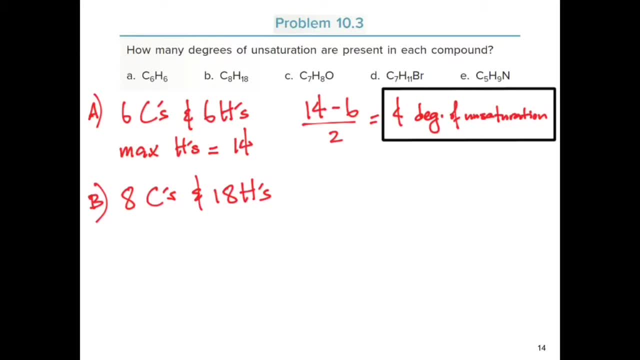 And to get the maximum here we multiply the number of carbon atoms by 2, and then add 2.. So we have 8 times 2 equals 16, plus 2 equals 18.. So we already have the maximum number of hydrogen atoms. 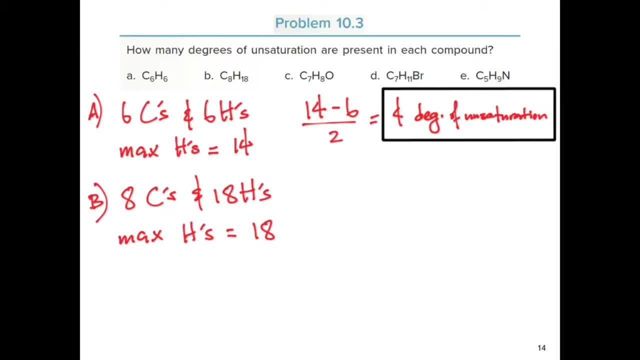 for this specific molecule And for part C. here we have C7, H8, O, So we have 7 carbon atoms, 8 hydrogens and 1 oxygen. And so with oxygen atoms we can just ignore them because they don't play a part in the degree of unsaturation. 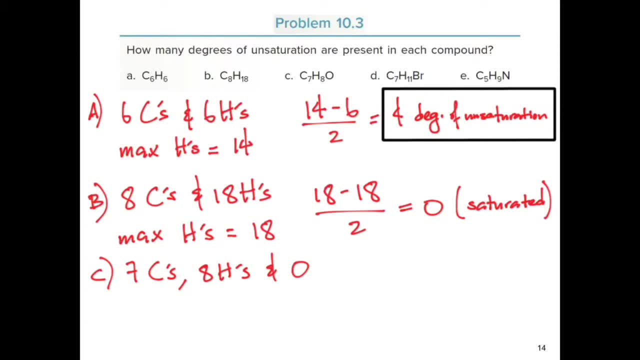 And so the maximum number of hydrogen atoms here is 7 times 2 is 14, plus 2 equals 16.. So 16 maximum hydrogens. Subtract that by 8, and divide it by 2, and we get 4 degrees of unsaturation. And for part D, here we have C7, H11, Br, So we have 7 carbon. 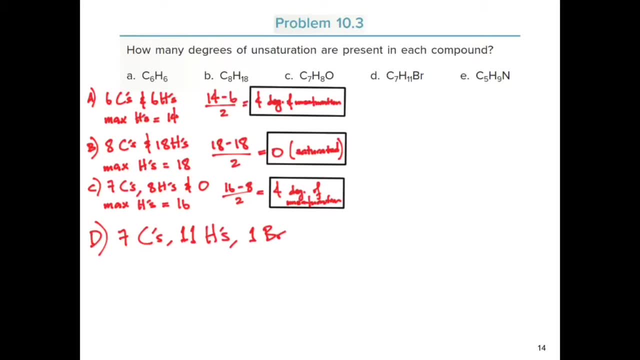 atoms, 11 hydrogen atoms and 1 bromine. And so in order to calculate the maximum number of hydrogens here, we multiply 7 by 2.. So 7 times 2 is 14.. So we have 6 maximum hydrogens that are clung to the Окra And the maximum amount you can add to this. 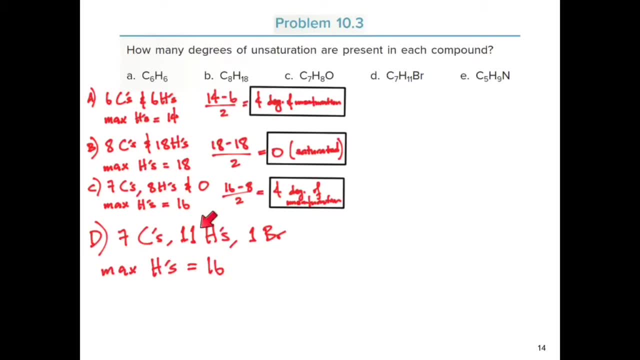 is 12. And so we've got 11.. So add it up to the remaining 16.. And then we're going to subtract, or we' were going to add 11 and 1, because bromine basically counts like a hydrogen atom. 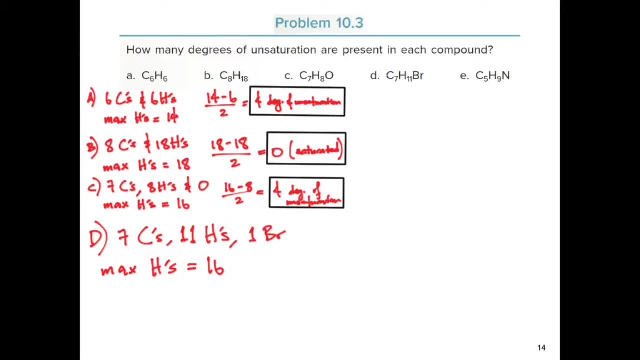 So 11 plus 1 is 12.. Subtract 12 from 16 and divide that by 2, and we get 2 degrees of unsaturation. And then finally we have C5, H9, and 1 nitrogen, So we have 9.. We have 5 carbon atoms, 9 hydrogen atoms. 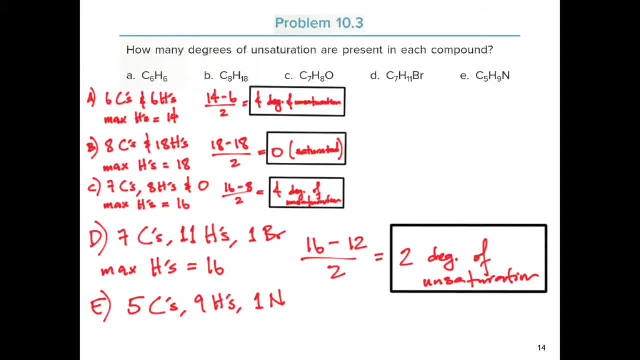 and 1 oxygen and one nitrogen, So the maximum number of hydrogens here is 12.. And then we're gonna subtract one from nine, because nitrogen- we have to subtract one from hydrogen for every one nitrogen, And so in that case we have eight hydrogens here. 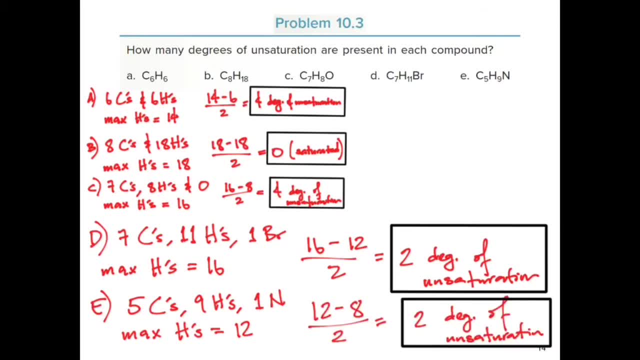 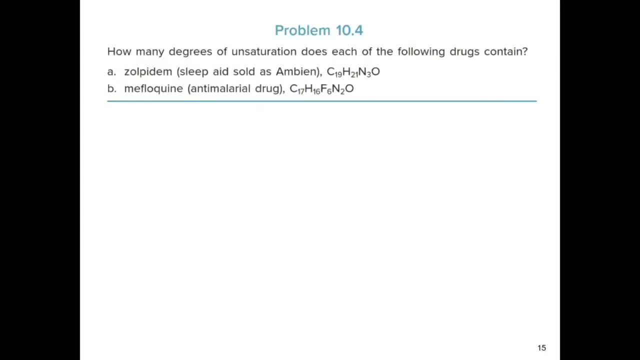 So 12 minus eight is four. and divide that by two and we get two degrees of unsaturation. And here's another practice problem: How many degrees of unsaturation does each of the following drugs contain? So the first one here is Zolpidem. 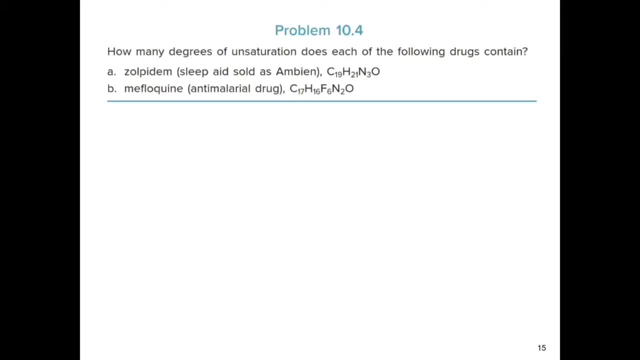 which has the chemical formula C19H21N3O. So we have 19 carbon atoms, 21 hydrogens, three nitrogens and one oxygen, And so the maximum number of hydrogens possible here would be 19 times two plus two equals 40.. 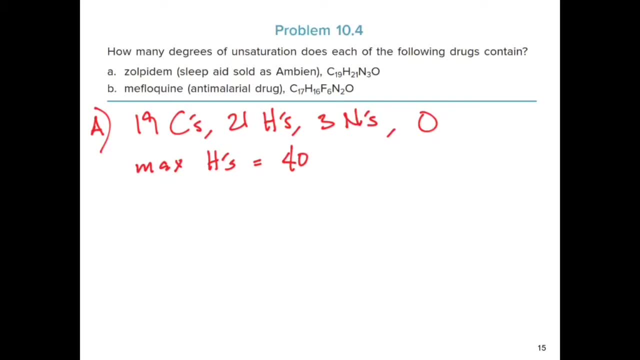 So we have 40 maximum hydrogens possible And to calculate the degrees of unsaturation, we're gonna subtract 21 from 40, as shown here. So we're also subtracting three nitrogens because, again nitrogen, we have to subtract one. 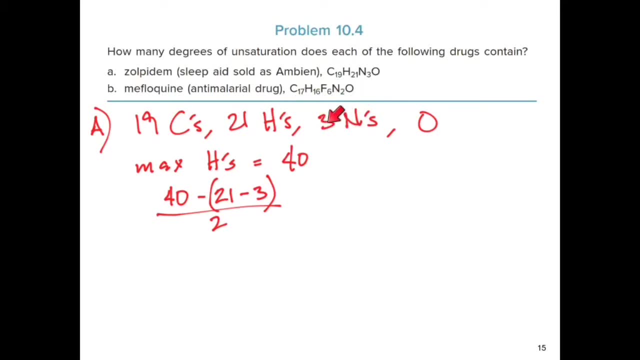 from hydrogen for every nitrogen present. And so, since we have three, we're gonna subtract three from 21, and then subtract that from the maximum, which is 40. So, in this case, 40 minus 21, minus three, divided by two. 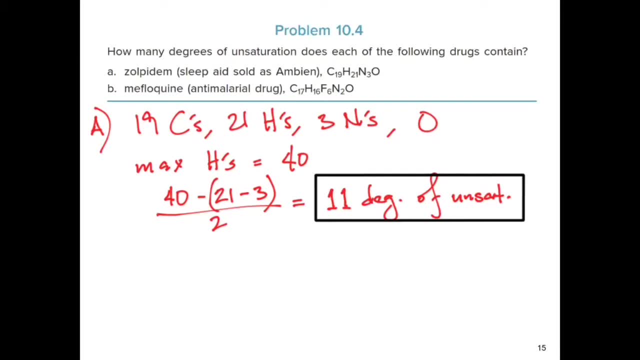 and we get a total of 11.. So this is 11 degrees of unsaturation. And for the second one, here we have Mifloquine, which has the chemical formula C17H16F6N2O. So we have 17 carbon atoms, 16 hydrogens. 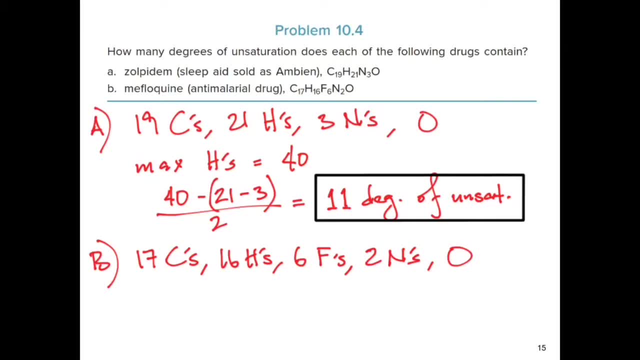 six fluorines, two nitrogens and one oxygen. So the oxygen we can just ignore that. but we have to subtract two nitrogens from 16 hydrogens and then add six fluorines, because fluorines basically count like hydrogens. 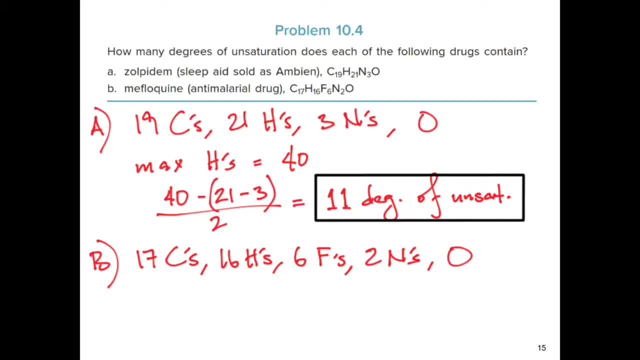 And so the maximum number of hydrogens here is 36.. 17 times two plus two equals 36.. And then calculating the degrees of unsaturation, here we're gonna subtract the maximum or take the difference between the maximum and the number of hydrogens. 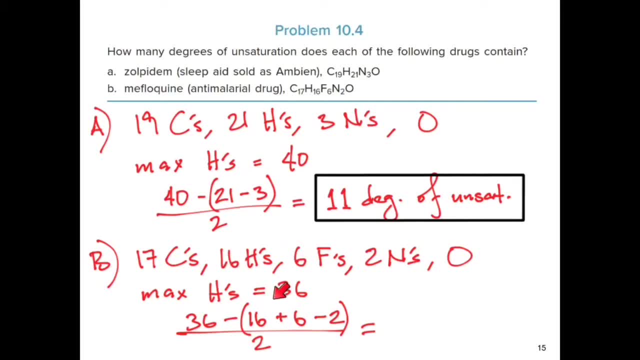 So again we have 16 hydrogens. We're gonna add six because of the fluorine atoms And then subtract two because of the nitrogens, And then subtract all of this from this from the maximum, and divide that by two and we get eight degrees of unsaturation. so now let's. 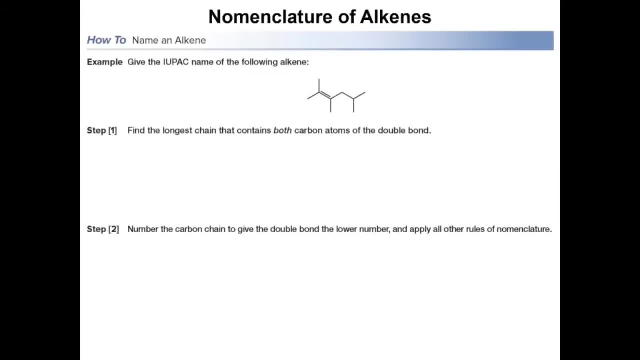 take a look at the rules regarding naming alkenes. so how do we name an alkene using the iupac system? so here's an example. you can see that we have a double bond here between these two carbon atoms, and the very first step here is to find the longest chain that contains both the carbon atoms. 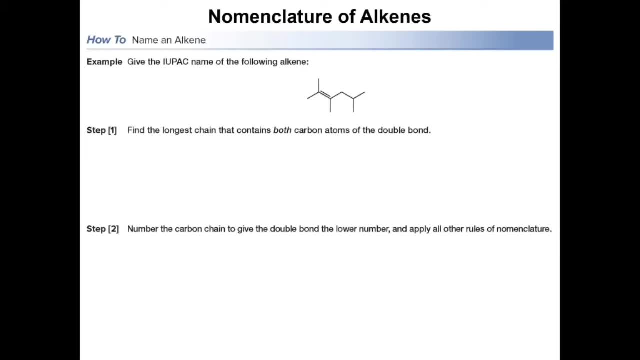 of the double bond, and so in that case our longest chain here would be this one right here. all right, so count the total number of carbon atoms here. we have one, two, three, four, five and six. so that means that we're going to have a hex scene here because of six carbon atoms. 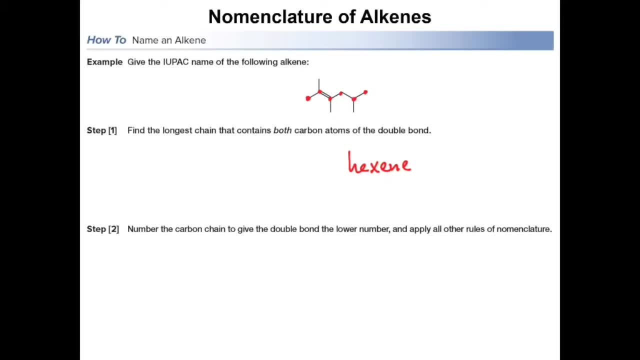 and then step number two here says: number the carbon chain, to give the double bond the lower number and then apply all the other rules of nomenclature and so the. So the double bond is right over here, and so we're going to label the carbon atoms from: 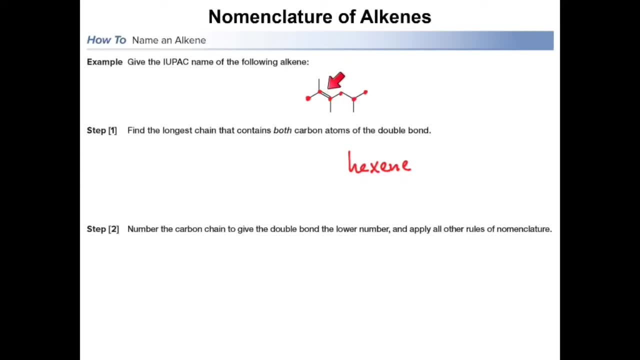 left to right so that it'll give the double bond the lower number. And so we have one, two, three, four, five and six. So you can see that we have the double bond on carbons two and three. And so once you've numbered the carbon chain to give the double bond the lower number. 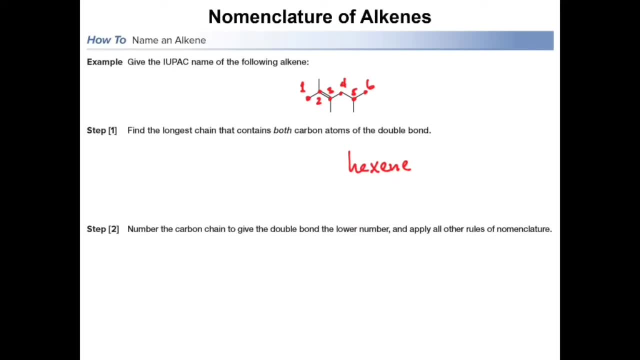 we're going to apply the other rules of nomenclature And so we're going to name this hex, and then the number two, and then E and E. So the number two here indicates that the functional group, the double bond, is on carbon. 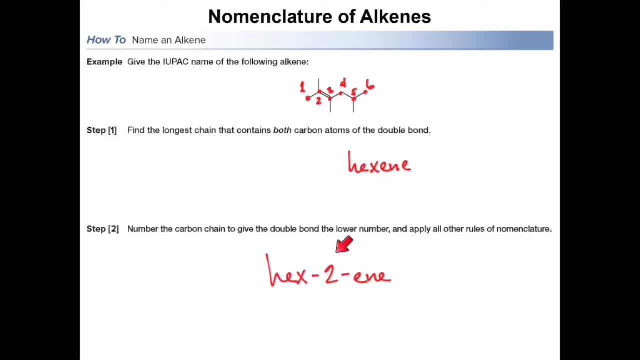 number two and three. So we're going to use the lower number, which is two instead of three, here in naming this alkene. So we have a hex to E and E or hex to E and E, And then, finally, we're going to name the substituents. 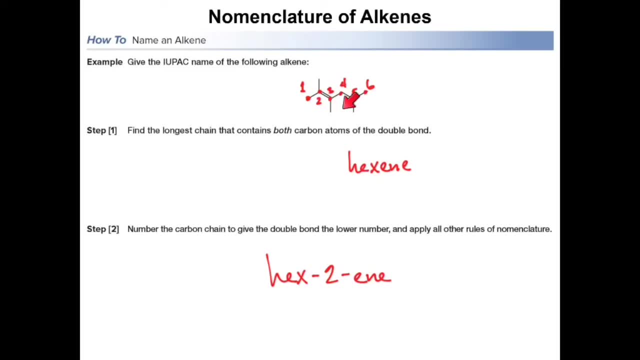 So you can see that we have one, two, three methyl groups here. So it's going to be on the second carbon atom, the third carbon and the fifth carbon atom. So we have a, two, three, five trimethyl. So that is two, three, five trimethyl. hex to E. 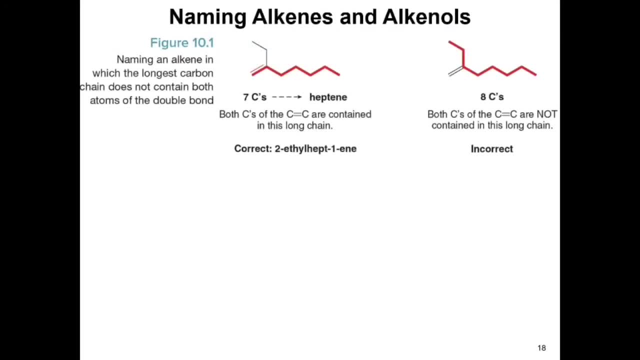 So whenever you're naming an alkene, you always want to make sure that whenever you're finding the longest chain to include both carbon atoms that are involved in the double bond. So, for example, over here, even though the longest chain contains eight carbon atoms, 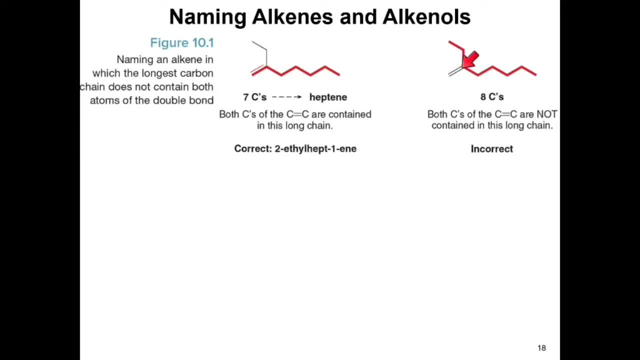 this would be incorrect because you didn't include both carbon atoms that are involved in the double bond. So the correct way to name this would be this one right here on the left, In which the double bond, or both carbon atoms in the double bond, are part of the longest. 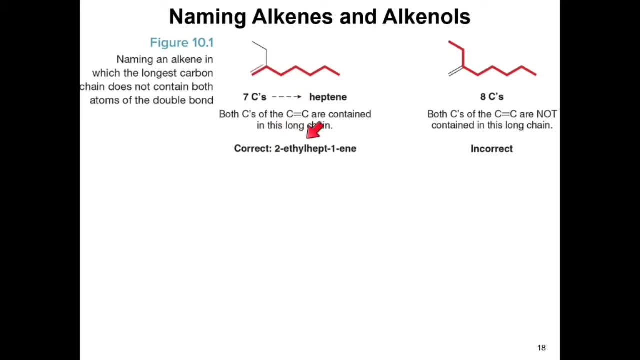 chain, And so the correct name for this is 2-ethyl-hept-1-ene. So again, that's 2-ethyl-hept-1-ene. So a lot of organic compounds can contain multiple functional groups, But compounds that contain both a double bond and a hydroxy group are called alkenols. 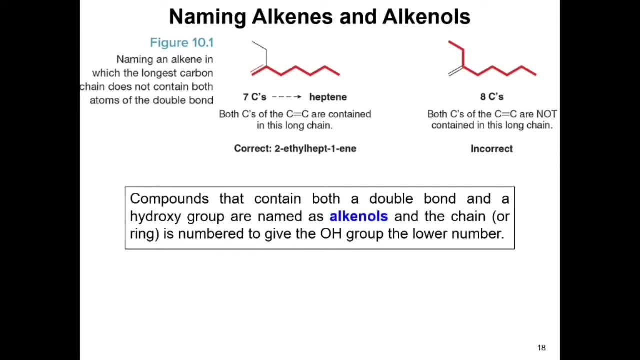 And the chain or ring is numbered to give the hydroxy group the lower number. So in that case the hydroxy group gets the higher priority over the double bond. So here are two examples of alkenols. You can see that they both end in enol. 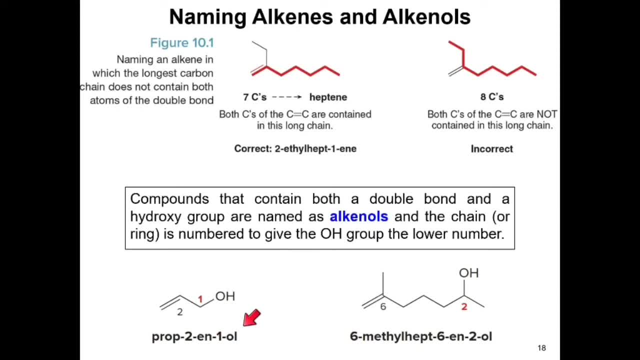 The suffix is enol, E-N-O-L, And the hydroxy group gets the higher priority, So it has the lower number, So it ends in 1-O-L, And then you can see that the double bond here is numbered 2, right. 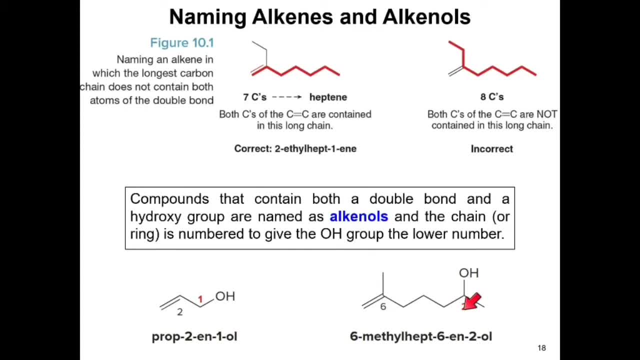 So it's 2-E-N-1-O-L. Same thing over here. You can see that the hydroxy group gets the higher priority, So it gets the lower number, And then the alkene group. the double bond here is on the 6-carbon atom. 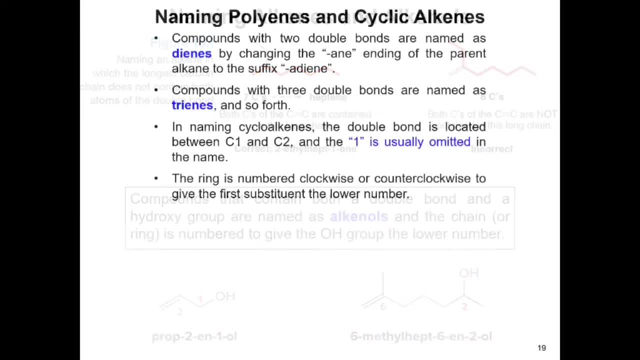 So that would be 6-E-N-2-O-L. So how do we name cyclic alkenes and alkenes containing multiple double bonds? So here are some of the rules that you can use whenever you're naming these type of alkenes. 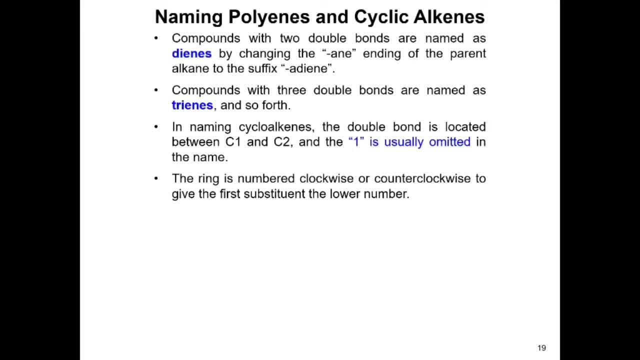 So the first one here says: compounds with two double bonds are named as dienes By simply changing the A and E ending of the parent alkene to the suffix adiene. Compounds with three double bonds are named as trienes, and so forth. 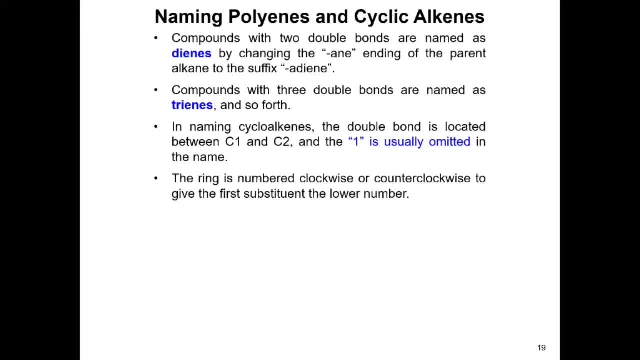 And in naming cycloalkenes the double bond is located between C1 and C2. And the one is usually omitted in the name because again you have a cyclic ring. The ring is numbered clockwise or counterclockwise, to give the first substituent the lower number. 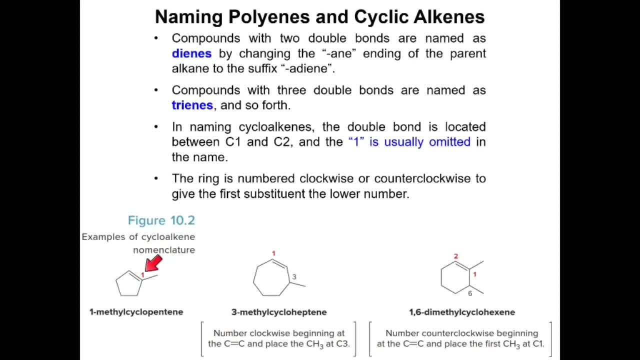 So let's take a look at a few examples here. Here we have a cyclopentene ring in which the first substituent is bonded to the first carbon atom, And so here we have one methyl cyclopentene And then the next one. here we have a cycloheptene with seven carbon atoms. 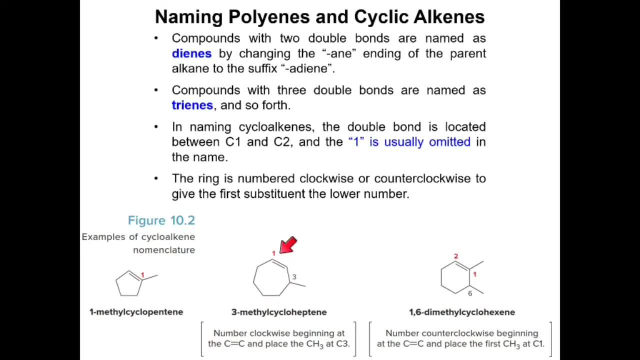 And again, the double bond is labeled as the first carbon, And so we're going to label the carbon atoms clockwise, to give the second or the first substituent here the next number, And so that would be 1,, 2,, 3.. 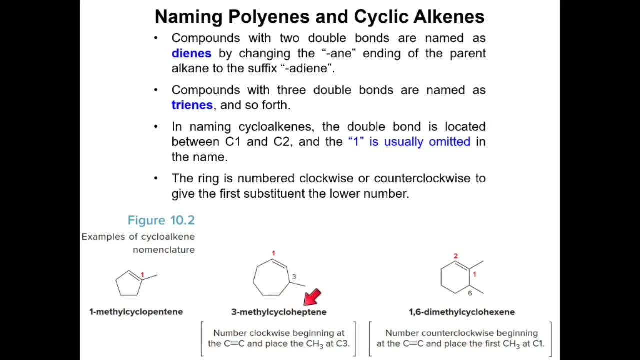 And so we have a 3-methylcycloheptene, And then for the third one here we have a cyclohexene, because we have a total of six carbon atoms in the ring. And then we're going to number the first metal group here as the first substituent. 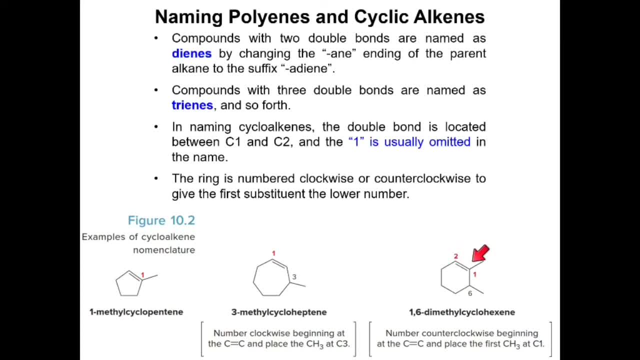 So we have 1, 2.. So we're numbering the carbon atoms counterclockwise this time. So that's 1, 2, 3, 4, 5, 6.. So we have a methyl group bonded to the first carbon atom. 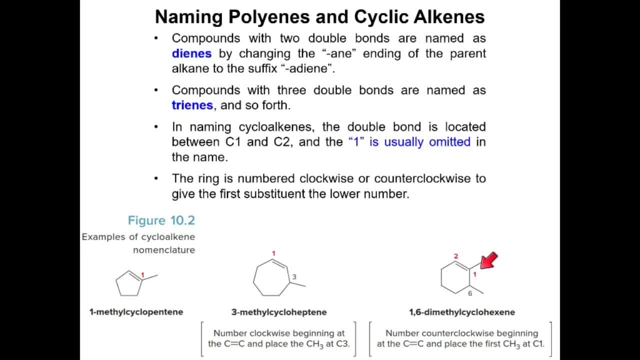 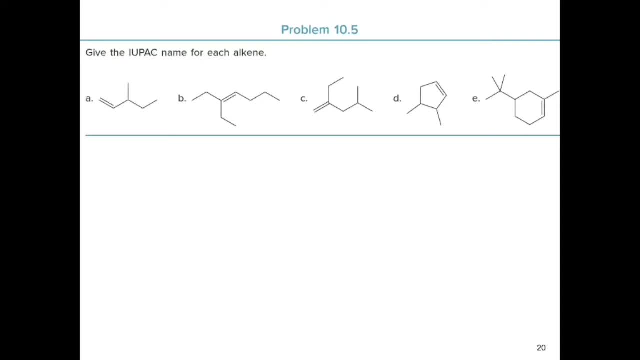 And another one on the sixth carbon atom. So when naming this ring, here we have 1, 6-dimethylcyclohexene. So here's practice problem number five: Give the IUPAC name for each alkene. 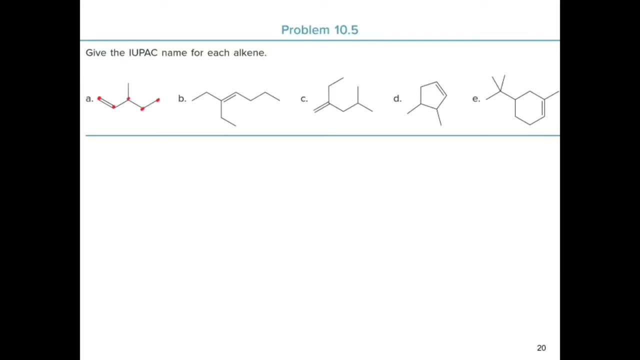 So for the first one here, we have this longest chain which contains five carbon atoms, including the double bond, And so this is going to be a pentene in which the double bond is on the first carbon atom. So this is going to be labeled from left to right. 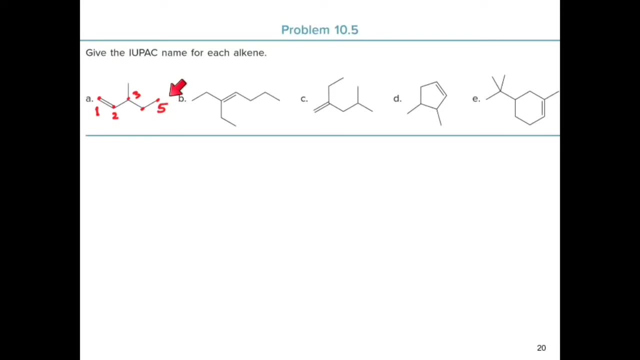 1,, 2,, 3,, 4, and 5, in which the double bond again is on the first carbon atom, And so this is going to be a pent-1-ene, And then you can see that we have a methyl group bonded to the third carbon atom. 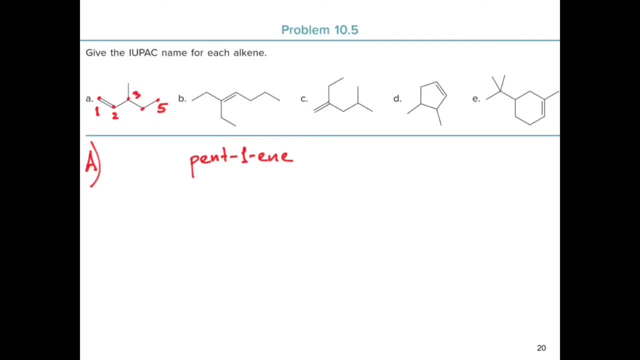 And so the compound's name is going to be 3-methyl-pent-1-ene. And for the second one- here, this is our longest chain. You can see that there's a total of seven carbon atoms Again, which includes the double bond. 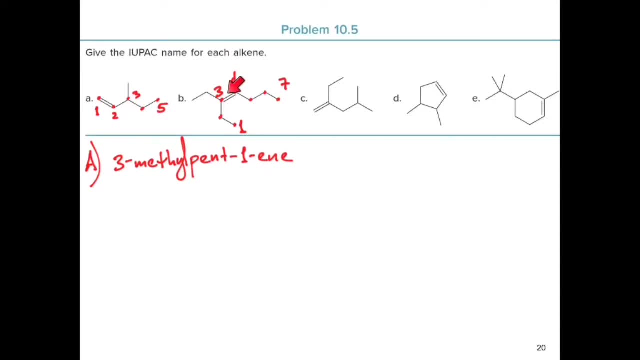 And the double bond is going to be on the third and fourth carbon atom. So again, you want to minimize the number of the double bond. So instead of counting from right to left, it's going to be from left to right. So in this case, since we have seven carbon atoms, this is going to be a hept-3-ene. 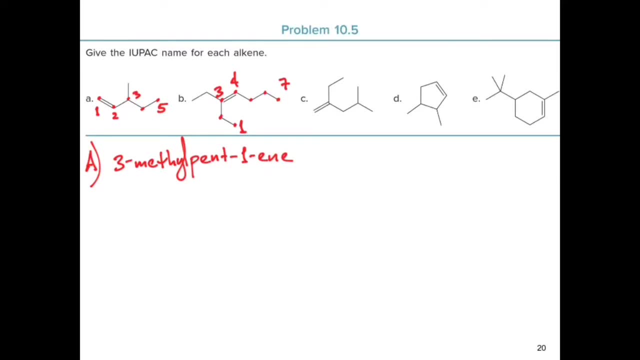 Hept-3-ene, And then, on the third carbon atom, this is going to be a pentene. On the third carbon atom, there's an ethyl group, And so in that case the name of this compound is going to be 3-ethyl-hept-3-ene. 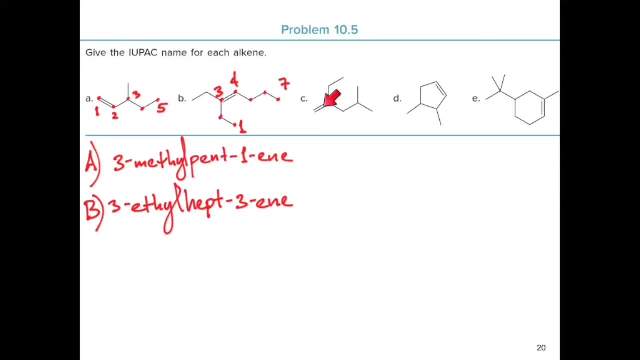 And for part C, here again we have to include the double bond, And so the longest carbon chain would contain one, two, three, four, five carbon atoms, And so the double bond is between carbons one and two, And so we're going to label this from left to right. 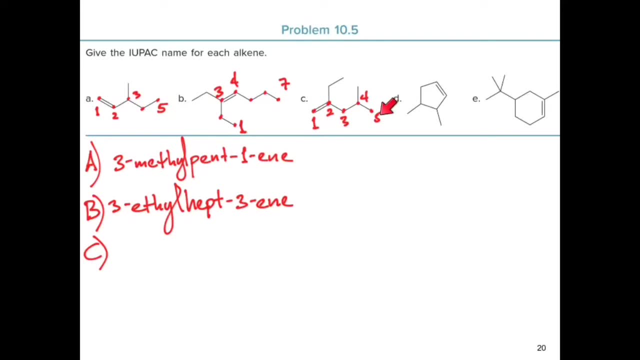 So in that case this is going to be a five carbon chain. So we have pent-1-ene, It's going to be a pentene, Pent-1-ene, And then you can see that we have a ethyl group on the second carbon and then a methyl. 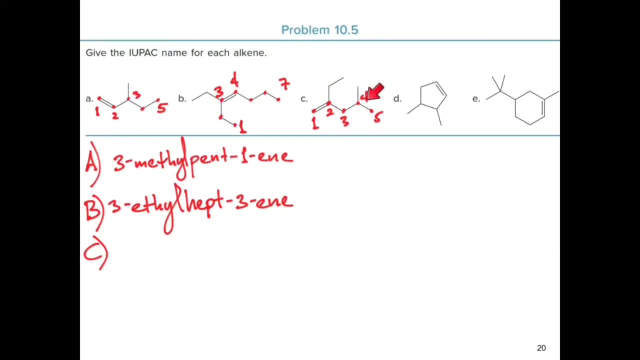 group on the fourth carbon, And so ethyl goes first before methyl, And so that's going to be 2-ethyl-4-methyl-pent-1-ene. For the fourth molecule, here you can see that we have ethyl-4-methyl-pent-1-ene. 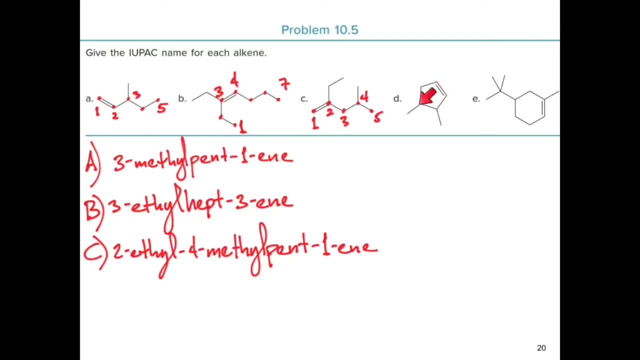 And so that's going to be 2-ethyl-4-methyl-pent-1-ene, And so this is going to be a cyclic ring containing five carbon atoms, And so this is going to be a cyclopentene, And we're going to label the carbon atoms clockwise, so that the first substituent gets. 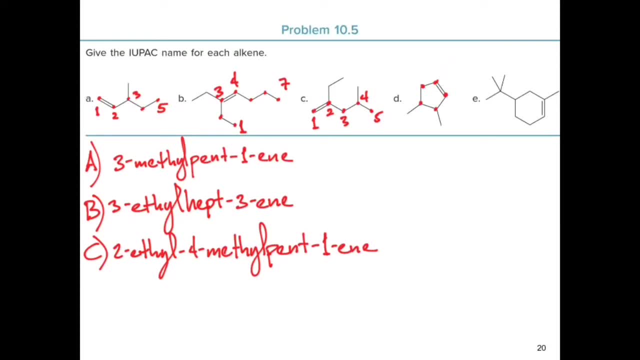 the lower number, And so, starting from the double bond, so we have one, two, three, four and five, And then notice that we have two methyl groups, one on the third carbon atom and another one on the fourth carbon atom. And so what we have here is 3,4-dimethyl-cyclopentene, And so what we have here is 3,4-dimethyl-cyclopentene, And so what we have here is 3,4-dimethyl-cyclopentene.